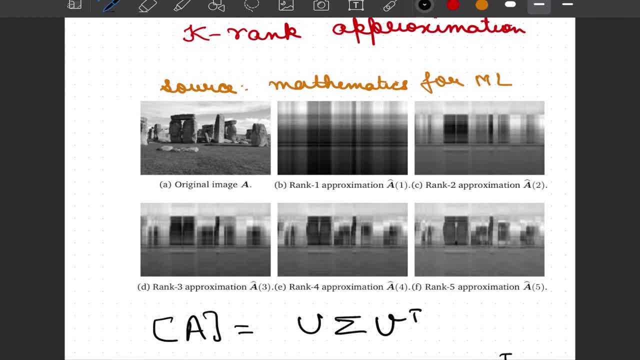 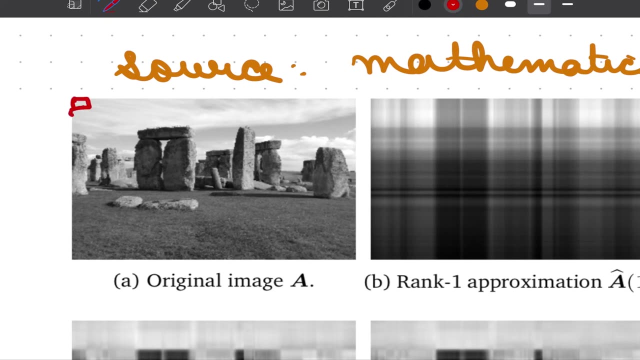 is basically number of independent vectors that we need to completely describe a vector space, and in the case of images, we are essentially dealing with the collection of data. so, for example, what we perceive as an image- you can always think of it- is like the collection of multiple pixels. 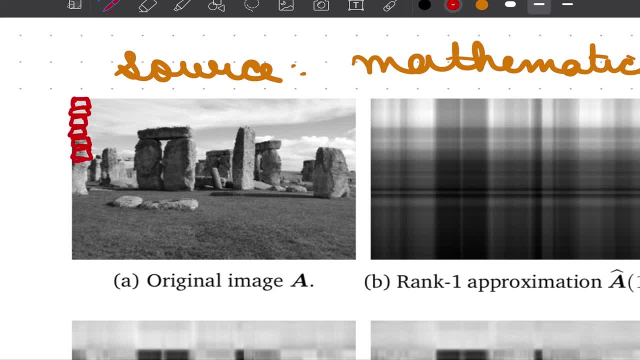 and each pixel is having some brightness value associated and if we are talking about our the, the, the, the the scale image, we can characterize this entire image using the intensity towards black or intensity towards white, and so on. So, basically, computer would see this image as the collection of numbers which are arranged. 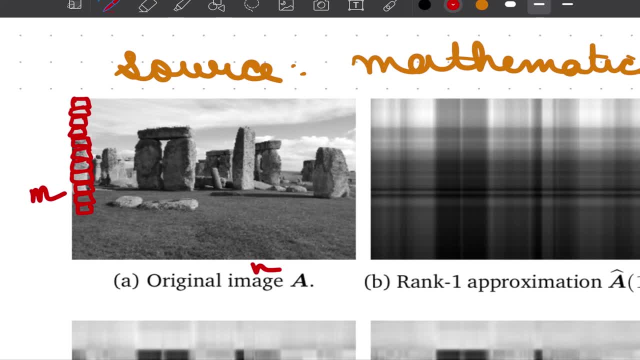 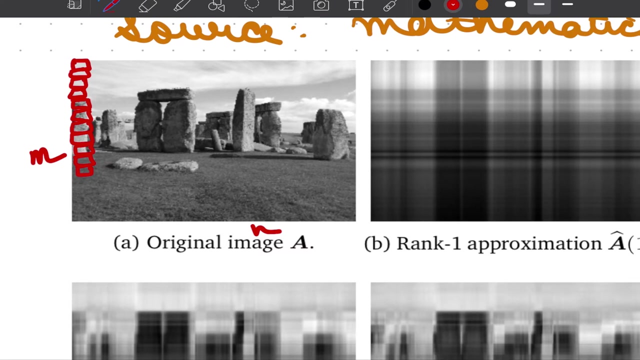 in some size of, let us say, m cross n. and now the question arises: do we really need entire information in this image to come up with some approximation, or there exists some concepts to which we can map this image and have a lower dimensional visualization? We also call this particular transformation, that is, from fine resolution image to coarse. 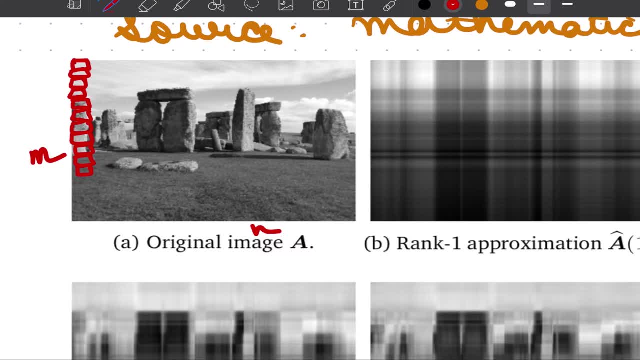 resolution image as the problem of upscaling In climate world. downscaling would mean we are going from a coarser resolution to finer resolution and the opposite would be upscaling, whereas in some domains the terminology is exactly opposite, where downscaling refers to getting a coarse version. 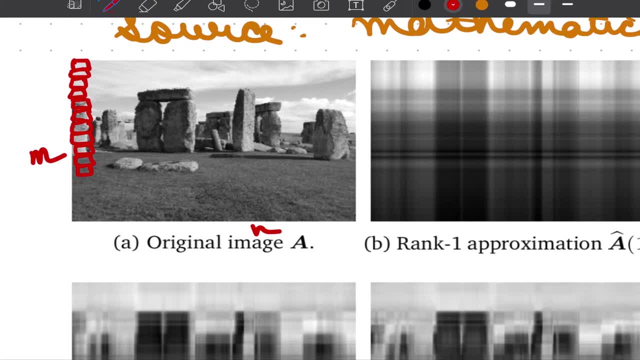 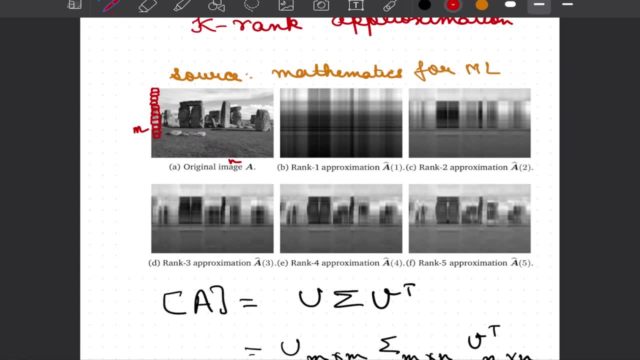 Whereas upscaling refers to the finer version. But the point here is that we want to reduce size of this image. we want to use less number of features and identify some concepts that can help us reconstruct this image. So what we do is that we try to come up with some approximations. that is the rank one approximation. 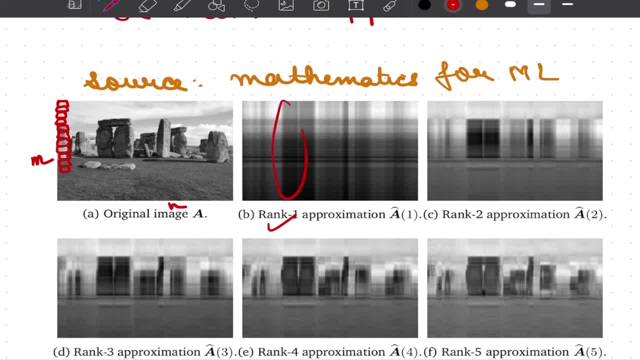 will try to capture some abstract feature. You see that there are certain bands. there are some horizontal bands as well as vertical bands. there are certain areas where the intensity of white patches is higher and so on. but you can clearly see that If you just look at rank one approximation, the lot of abstract features are captured. 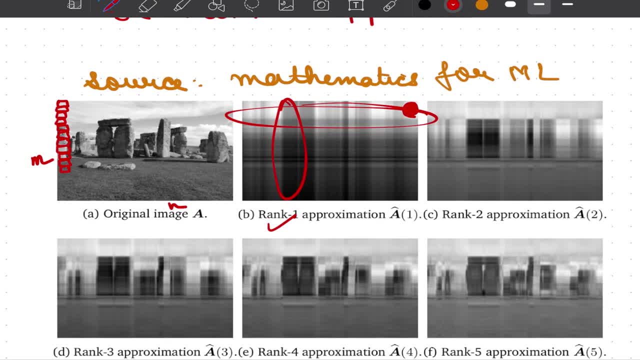 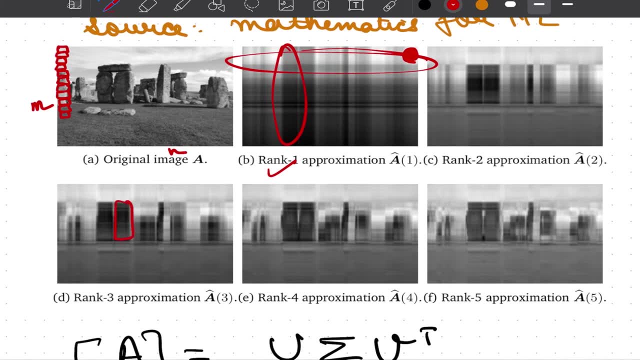 but it is nowhere closer to the image. Now, as we go towards the rank two approximation, or in fact rank three and rank four approximation, you see that the certain components of images is getting more clearer and clearer. Now you are able to detect some edges, you are able to discreetly identify some objects. 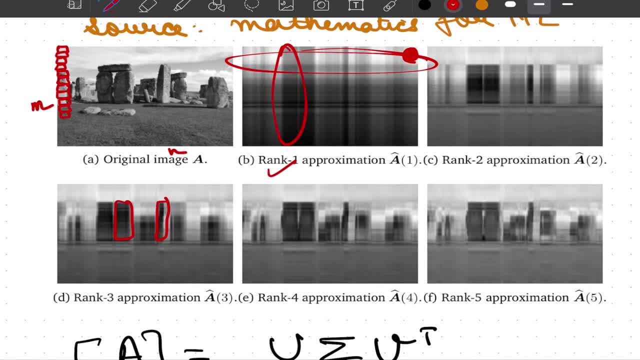 but you would never know whether that particular object is a tomb or it's a rock or it's something else. All you see is that some square form is combined And as we go towards higher approximation- that is rank four and rank five- it is becoming. 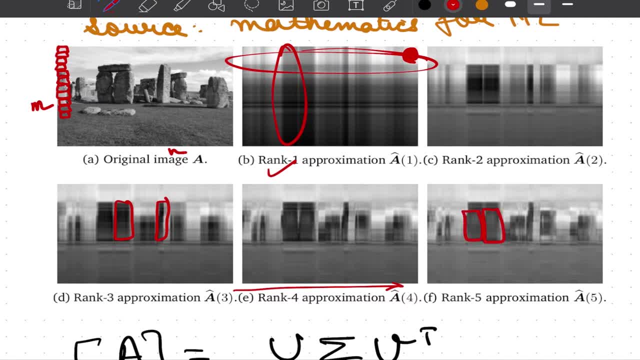 apparently clear that, yeah, this looks like. there are some images which look like rock, and here we may have a patch of grass and on top we may have a sky, but still not that clear. But still we can see that, as compared to original image, rank five approximation is taking us. 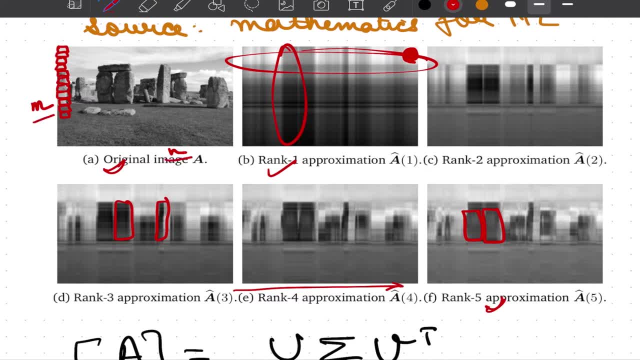 closer to the original image. Now, if these dimensions were in a few hundreds, let us say that m cross n Was of size, maybe thousand cross thousand. if we are talking about an HD image, we can really approximate it using m cross r representation, where r represents just the rank, five or 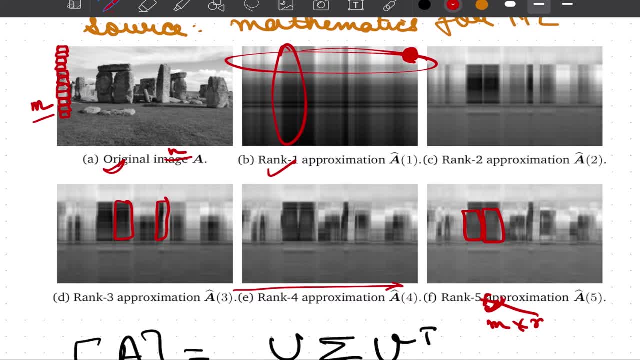 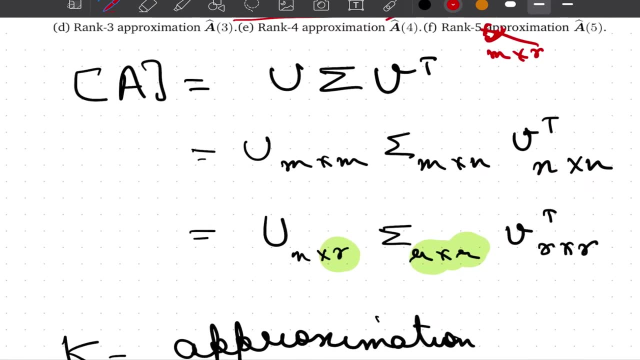 the or the thousand cross five approximation. that would basically convey the message without occupying too much memory space, And this also means that we have retained the meaningful information and able to reconstruct or get closer to our image. Again, you see that there is definitely going to be an error associated between a and the. 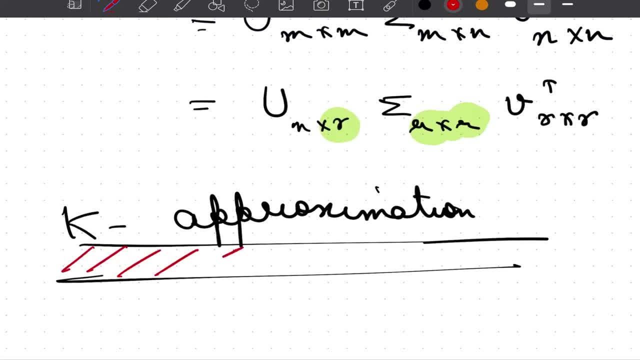 approximate image and we call this error as the difference between actual image, which we call as a minus, the k rank approximation of the same image. In today's lecture we will try to see that: how to come up with this k rank approximation and how to calculate losses. 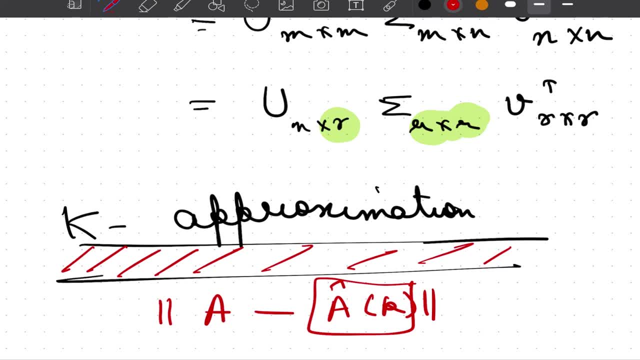 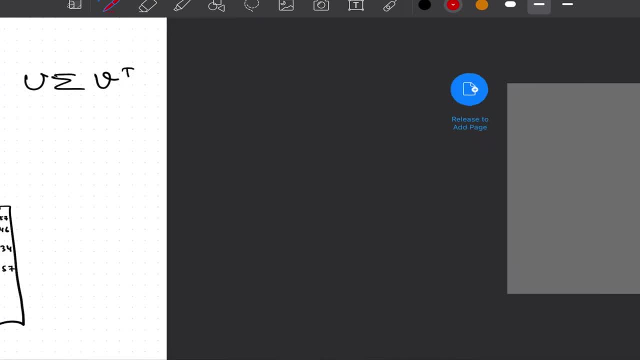 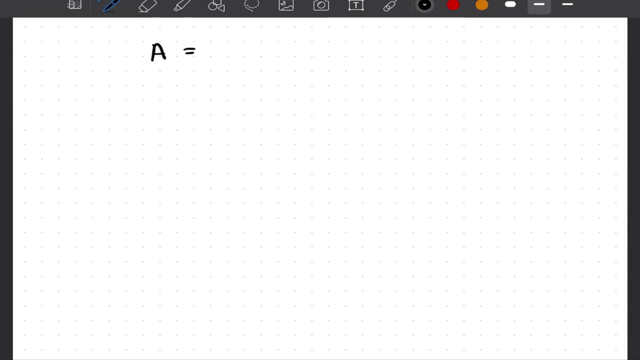 And what is the guarantee that this k rank approximation, derived using singular value decomposition, Is The Best approximation? Now we define the- we will come back to this example- but we define the k rank approximation as multiplication of i th column of our u, our u matrix that we get after SVD decomposition. 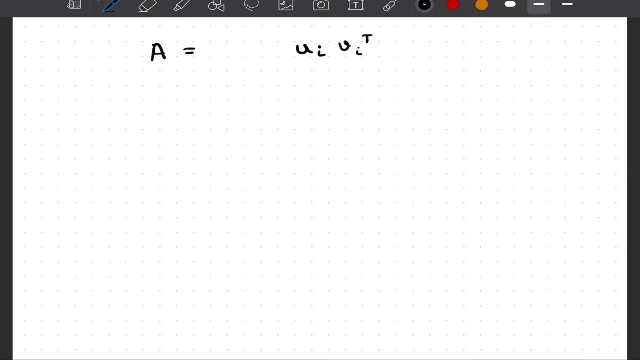 multiplied by the v i transpose, that would mean the i th row of v transpose, because we are already taking the transpose Multiplied, Multiplied by the scaling factor which is encoded in the sigma matrix. and if we are talking about the k? th approximation, we will take this i from 1 to k. 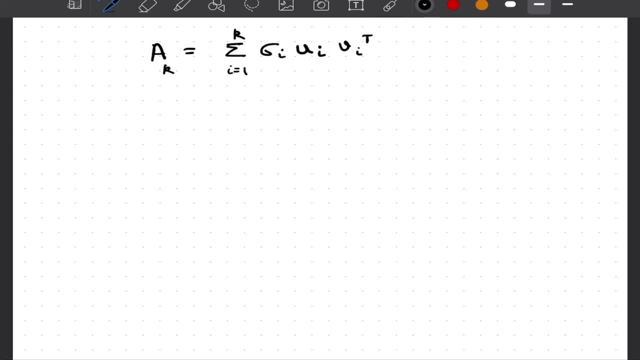 So that would mean that if we are interested in calculating fifth approximation, we can write this as: sigma 1 u 1 v 1- transpose, plus sigma 2 u 2 v 2- transpose, all the way till sigma 5 u 5 v 5 transpose. 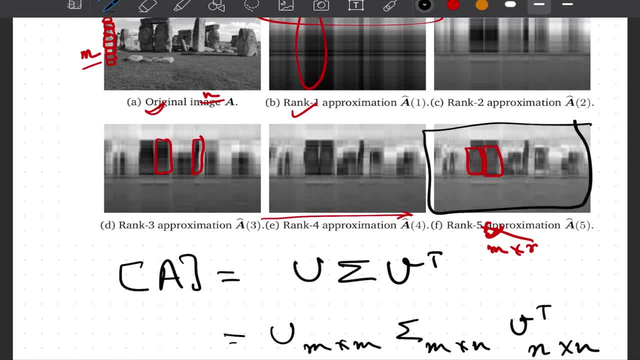 So this is how this fifth approximation that we saw in this image would have been derived. So what we will do, we will perform the singular value decomposition of whatever matrix we have. We will arrange our diagonal matrix in sigma, in descending order. So whenever we are talking about the k rank approximation, we are strictly saying that. 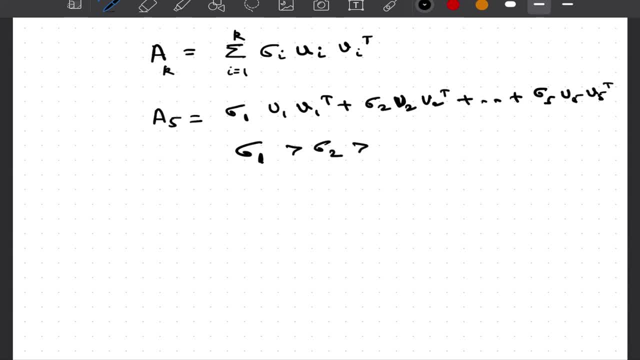 sigma 1 has to be greater than sigma 2.. Has to be greater than sigma 5, and if we are talking about certain cases where this could be 0. So we can say that sigma 1 has to be strictly greater than or equal to sigma 2, and so on. 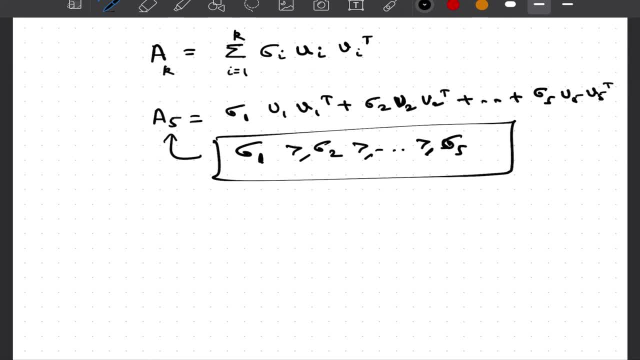 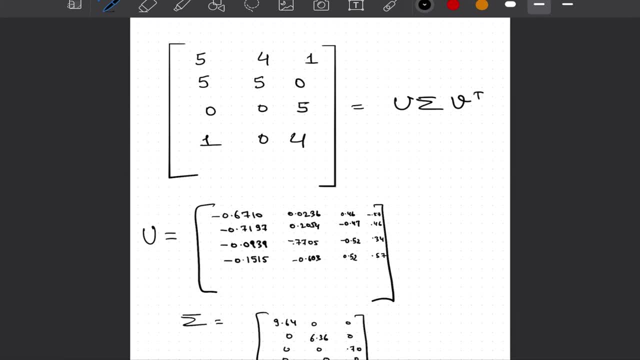 So under this condition, this will give us the k rank approximation. Now let us try to look this with the help of an example. This is the similar movie, matrix, that we discussed in our last video, but simplified Now what we do? we calculate its m cross, n decomposition. 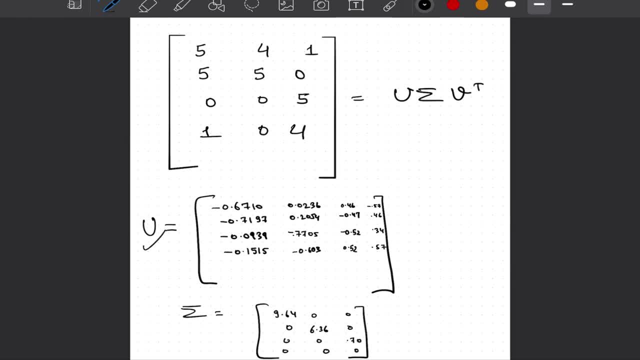 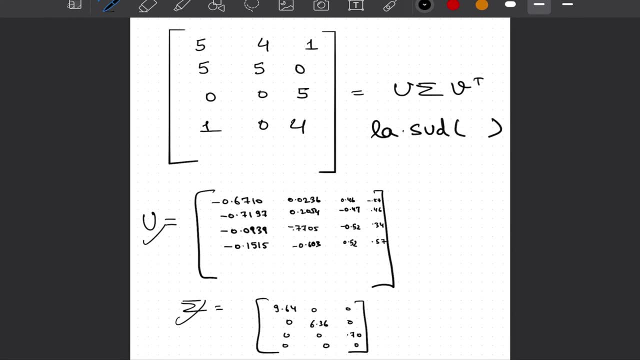 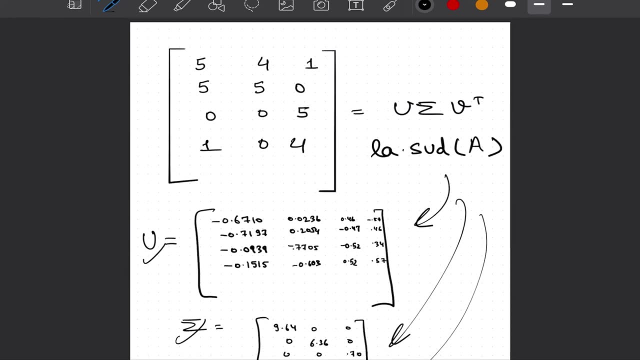 So u comes out to be this, sigma comes out to be this and v transpose comes out to be this Again. you can easily do this using the LA library in Python, which says that LA dot SVD of a should give us the components of u, sigma and v transpose. 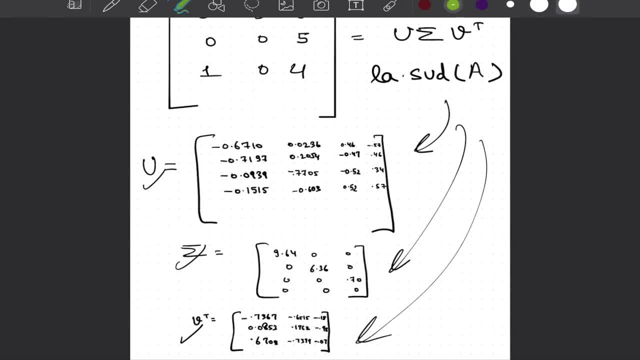 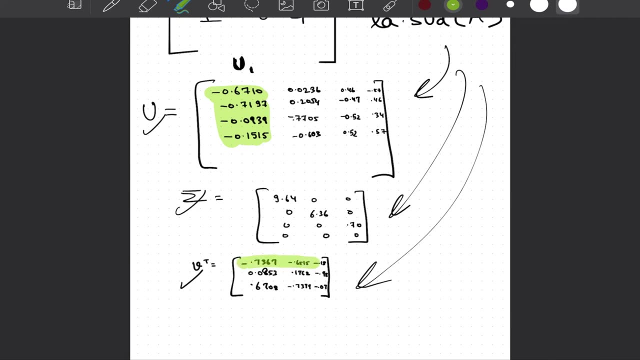 Now, if you have to calculate the first approximation, what we will do: we will take this value and the size of this vector. This is, this would be our u1. And we will multiply it by the transpose of v or the first value that is occurring here. 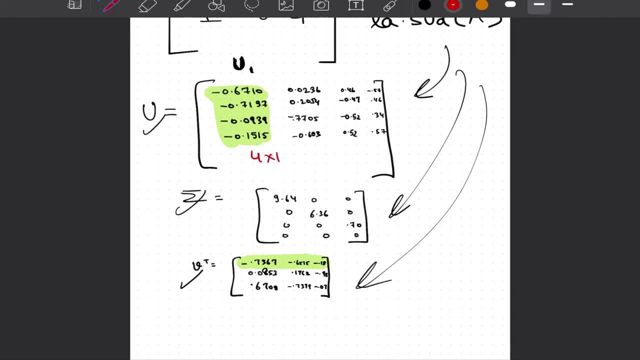 So basically, the size here is 4 cross 1, and we will multiply it by 1 cross 3.. So at the end we have the resultant size as 4 cross 3. And then we will multiply this particular transformation that we obtained, that is u. 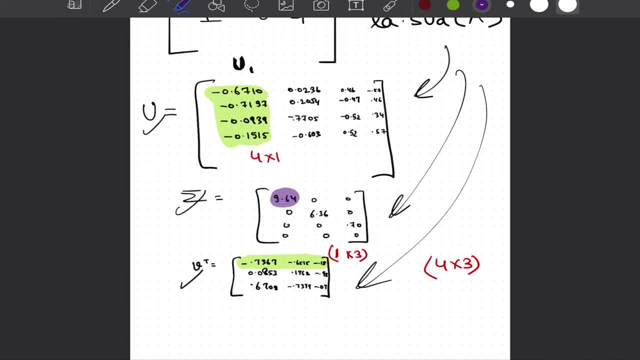 cross v by the first sigma. Now If we move to the second one, so let me color this also in gray: Now, if we move to the second one, we will take u2 multiplied by v2- transpose, and multiplied by this sigma, and we will add u1- v- transpose, sigma 1, plus u2- v2- transpose, sigma 2.. 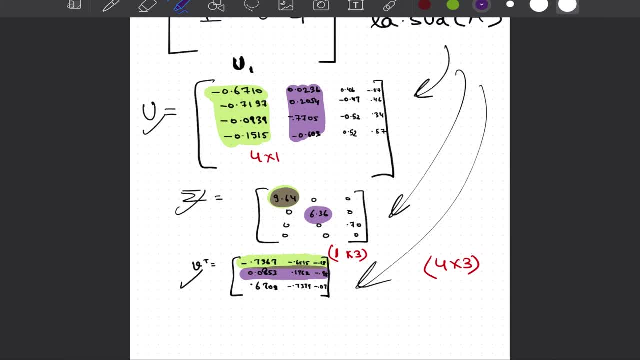 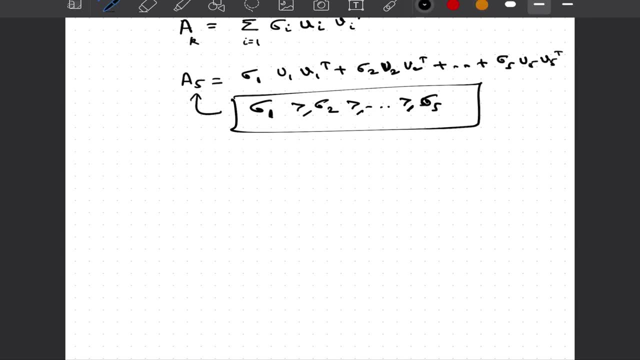 And if we are talking about rth approximation, we will keep on doing that until r sigma values, and that will help us reconstruct the image. Now the question arises: What is the mathematical guarantee that whatever approximation we are getting for that particular image is indeed the best approximation? 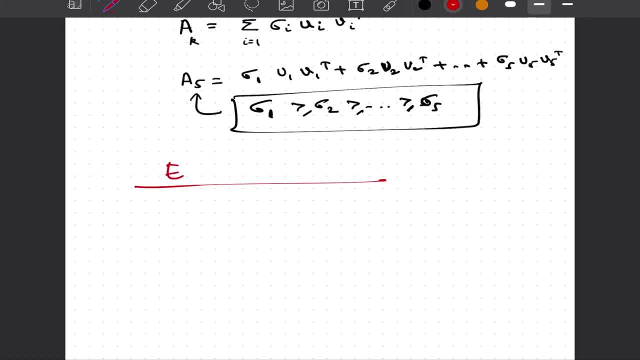 So we will not go into the theorems proof, But this is a famously known theorem as Eckart Young theorem. So Eckart Young theorem says that let us say that you have a matrix A and you come up with some k rank approximation as Ak. 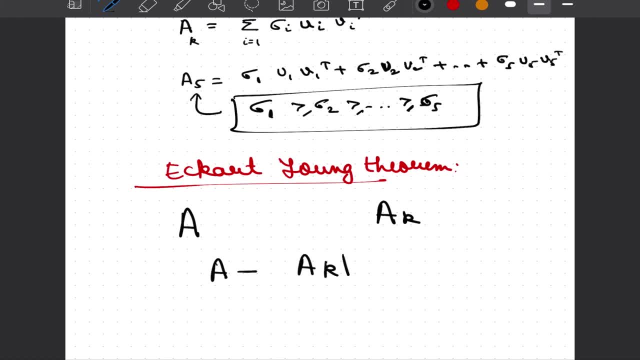 Then There should be some error associated with that k rank approximation. And if we are talking about here in case of matrix, we talk about these are the spectral norms. So what we learned about as the norms in the case of vectors, same thing concept can be. 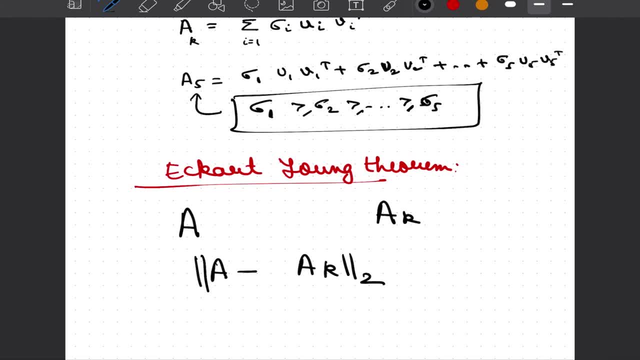 applied, but the name here becomes the spectral norm and the definition is said to be that spectral norm of A2 is defined as whatever, Whatever, Whatever maximizes the multiplication of AX or the L2 norm of of this multiplication multiplied by the L2 norm of the X vector, and wherever we find the maximum X, that is. 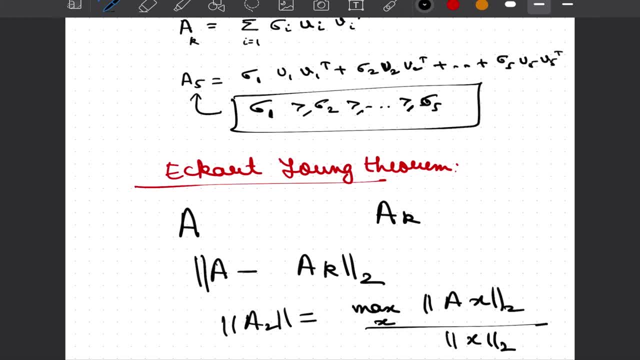 defined to be the spectral norm. But right now we should consider the spectral norm, rather than worrying about its mathematical complexity, as measure of some distance. So this is some measure of deviation. So So if the matrices are identically, are exactly identical, they are spectral distance should. 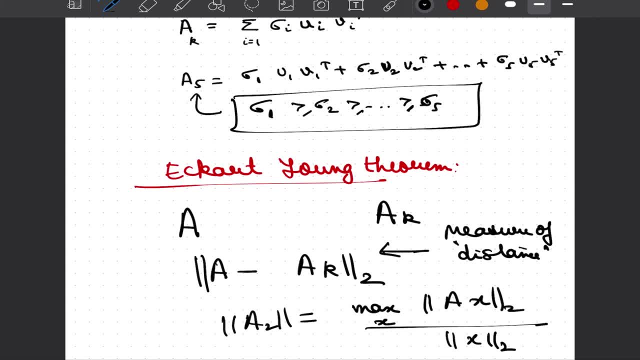 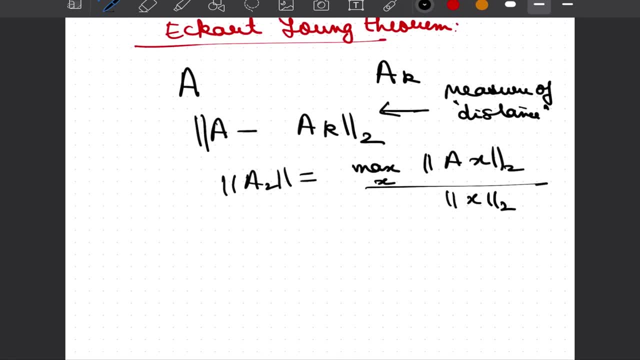 be equal to zero, or spectral norm should be equal to zero. That is a minus a k would tend to zero, And if they are very dissimilar from each other, they have to be. this has to be a larger number and that's the interpretation of the spectral norm also.